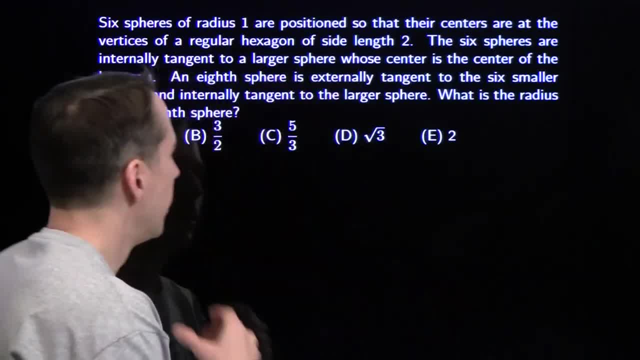 at the top of it. it's going to touch this larger sphere, All right, so we have at least somewhat of a picture of what's going on here, And we want the radius of this last sphere that we dropped in at the top there. Now one thing I like to do with these 3D problems. 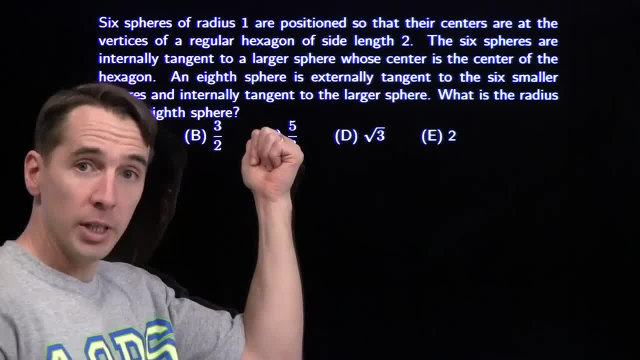 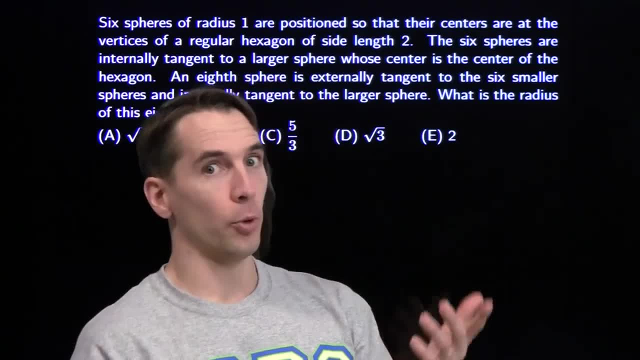 is. I like to take 2D cross sections, turn 3D problems into 2D problems And when I have a problem with a whole bunch of spheres, I like to throw my cross sections through centers of those spheres and through points of tangency, whenever I have tangent spheres- Now a natural 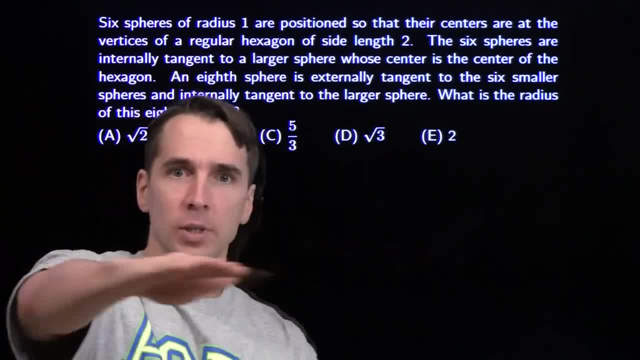 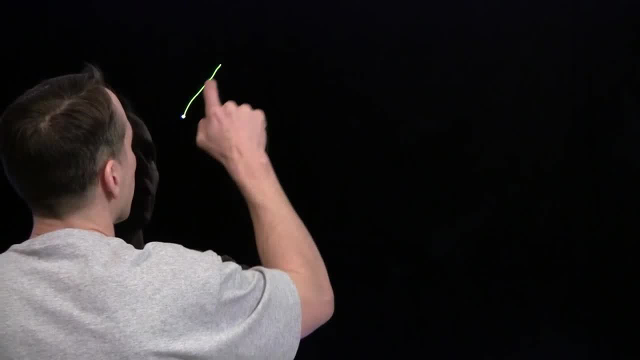 place to start here, of course, is the hexagon. We take the cross section with the hexagon because that's going to go through the centers of seven of these spheres and all kinds of points of tangency. So to start off, we'll draw a regular hexagon And you're going to 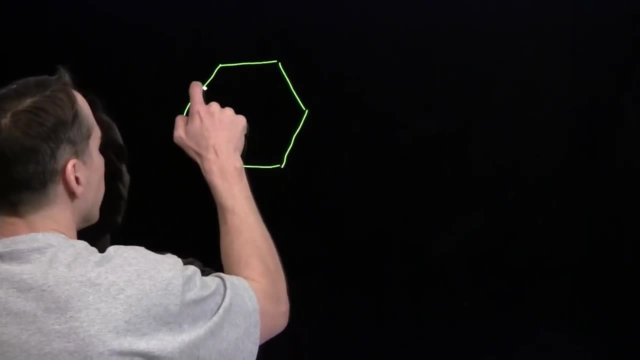 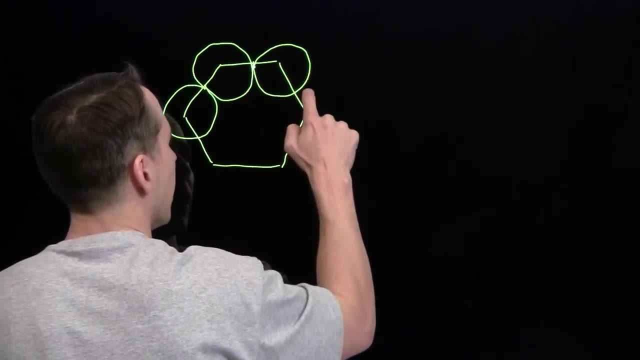 have to bear with me On the test. of course you've got your, you've got your ruler, you've got your protractor, you've got your compass, so you can draw a perfect diagram. You can probably draw a freehand better diagram- better than I can too. But when we take cross sections, 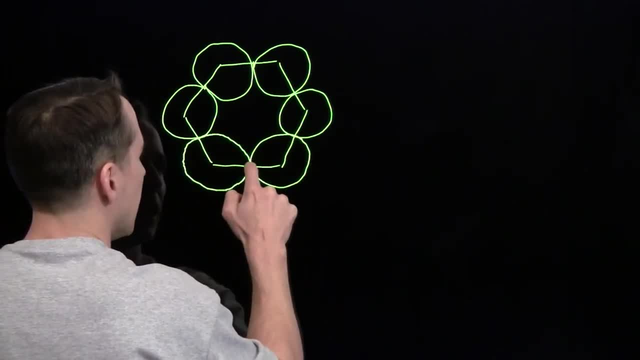 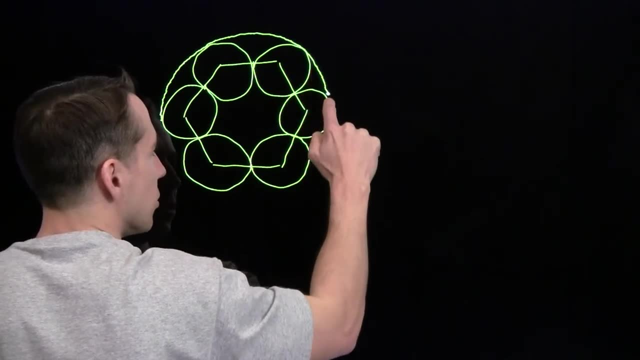 of our spheres. we make circles and we include the points of tangency in this cross section. Of course, we're also going to get the big sphere. The cross section of that is a circle that touches each of these little circles. All right, and there we go. This is the cross. 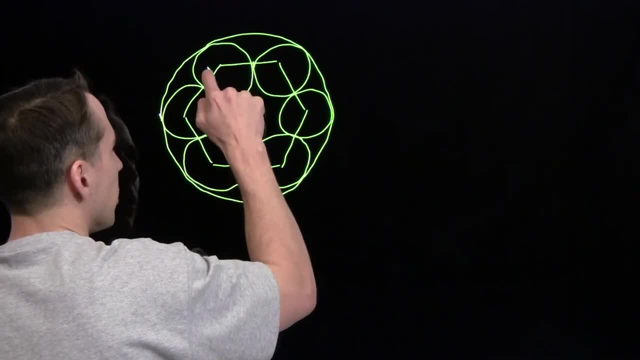 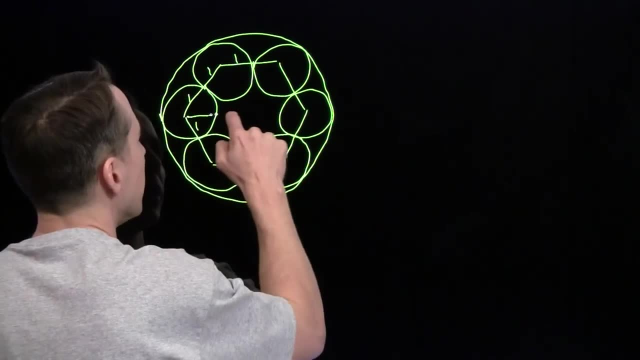 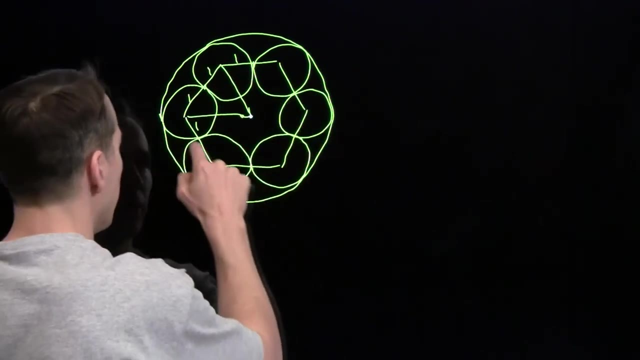 section through the hexagon. Now we can label some lengths. We know that the radii of the little spheres is 1. And one thing that's really nice about regular hexagons is you can break them up into equilateral triangles. So this is an equilateral triangle. Here's the center of the hexagon, center of 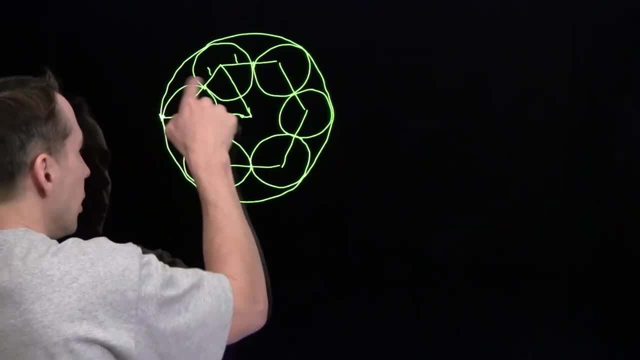 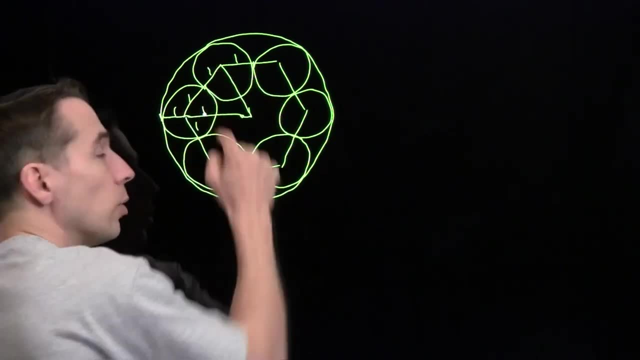 the big circle, And I can extend this out to the point of tangency of the small of this small sphere and the big one. So we know that this is 1, because it's the radius of the small sphere. This is 1.. This is an equilateral triangle, So this side is the same as this. 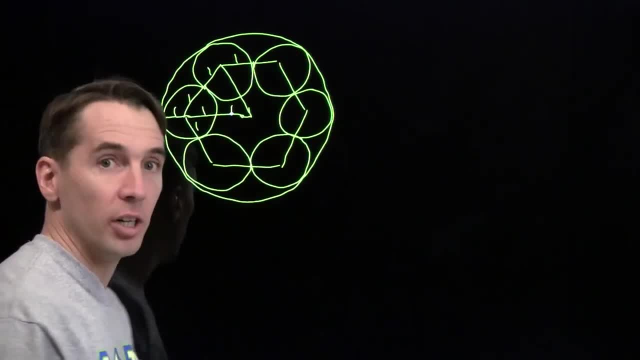 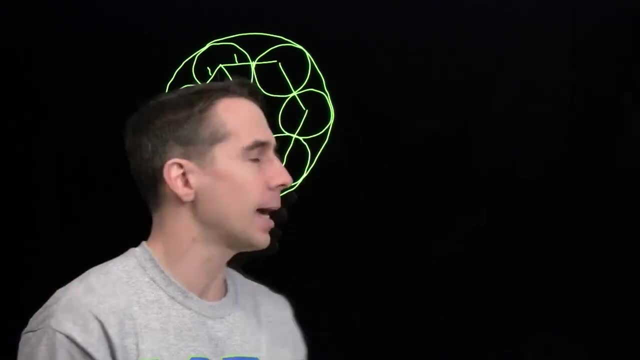 side. So it tells us that this is 1.. And now we know that the radius of the giant sphere is 3.. We've got the radius of the giant sphere. We've got the radii of all these little spheres. All we have left is that 8th sphere. we sat on top. Now, of course, that sphere is not. 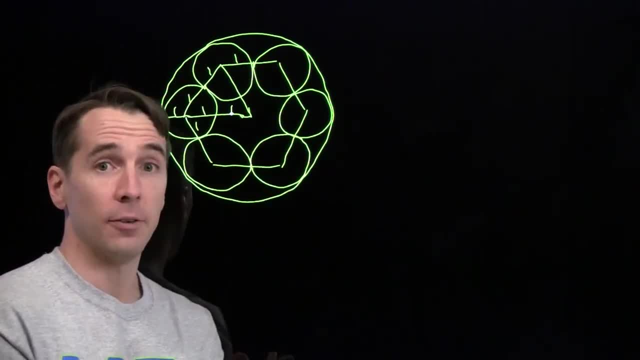 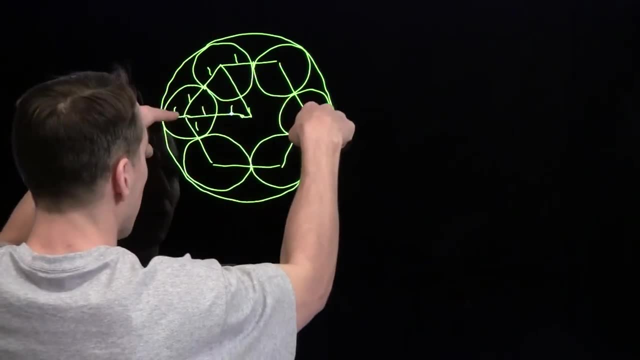 in this diagram. It's sitting right up here, So we're going to need a different cross section to go after this sphere. Of course, we're going to choose one that's going to go right through the center of that sphere. We want to hit some points of tangency. We want to 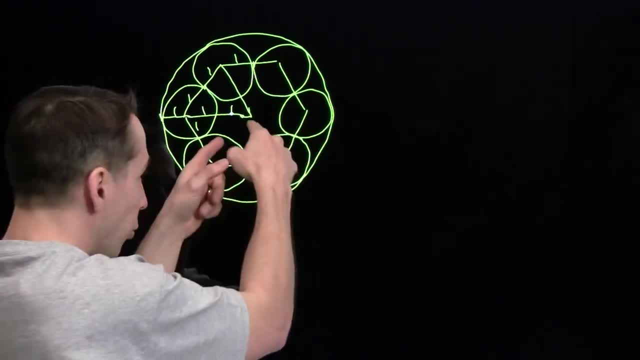 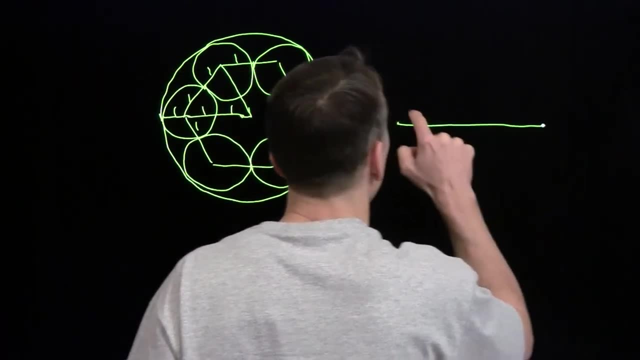 go through the centers of some of these little spheres and, of course, the center of our whole diagram, center of the big sphere. So we're going to take that cut right here And that cut's going to look like this: Got our little sphere. 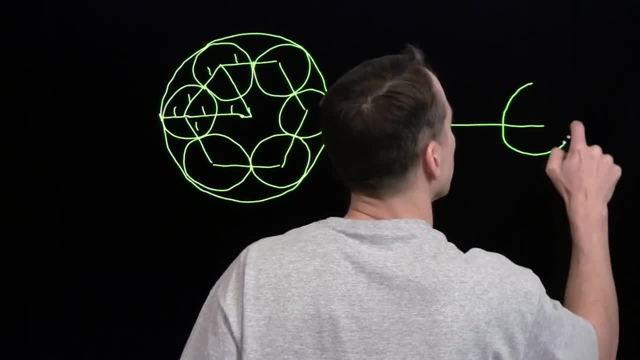 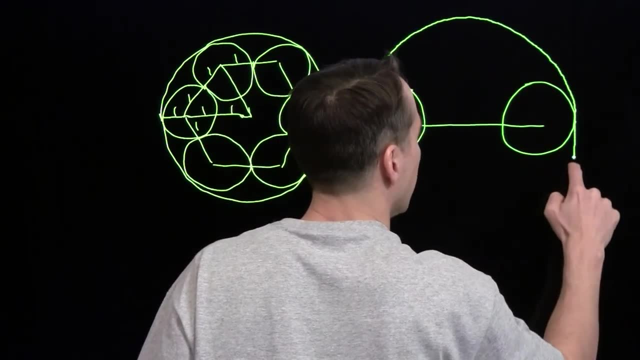 Got our little spheres out here still, And then we've got our big sphere that we just found has radius 3.. I'm not going to worry about what's going on down here, because then it won't be as embarrassing how badly I draw circles. 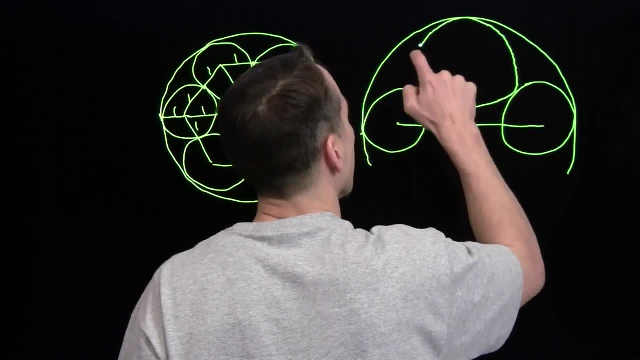 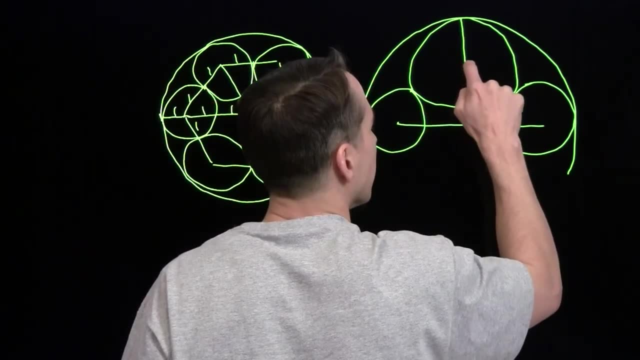 And then I've got another circle- This is my 8th sphere- this egg-shaped thing That's a circle. You have to use your imagination. This is the circle whose radius we're trying to find right there. That's the radius we want. Of course, we're going to continue this. 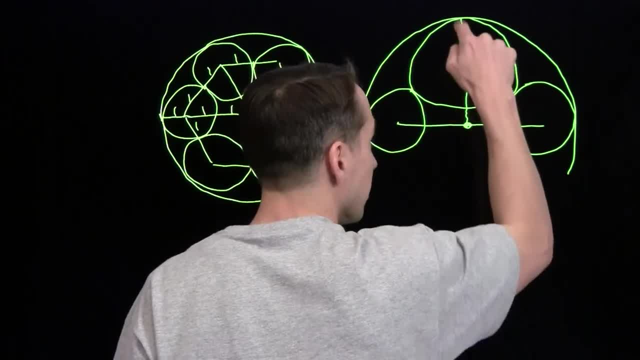 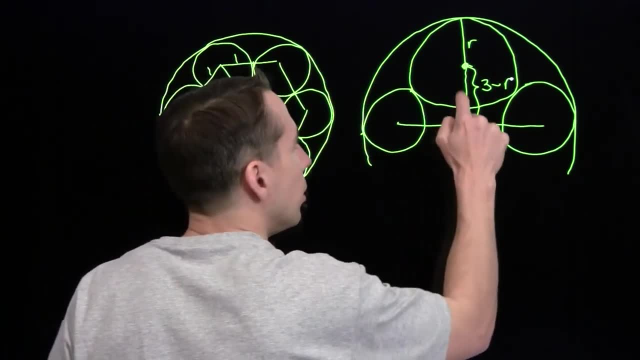 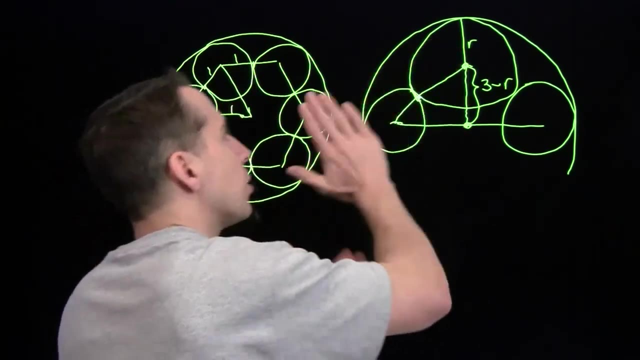 down to the center of the big sphere. And we know that this length, this is r, we know that this length is 3 minus r. And well, we can build a right triangle right here And you're going to have to use your imagination, but this cross section goes through the point. 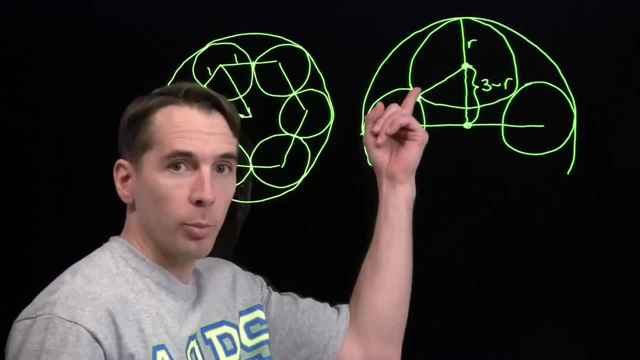 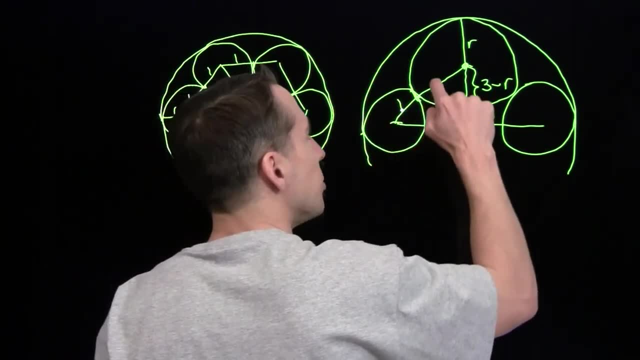 of tangency and these two centers. When we connect these centers, we go through the point of tangency. That's why, whenever we have two tangent circles, we like to connect the centers. We know that this is one, because this is one of our small spheres. 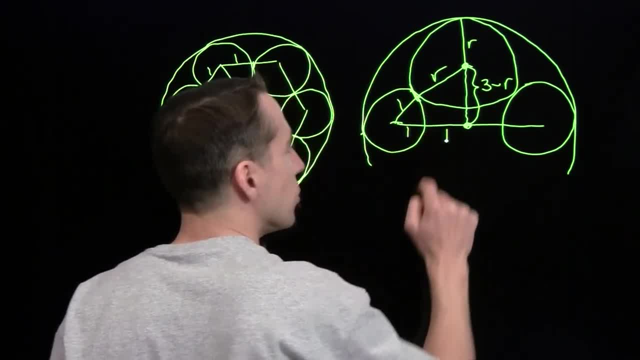 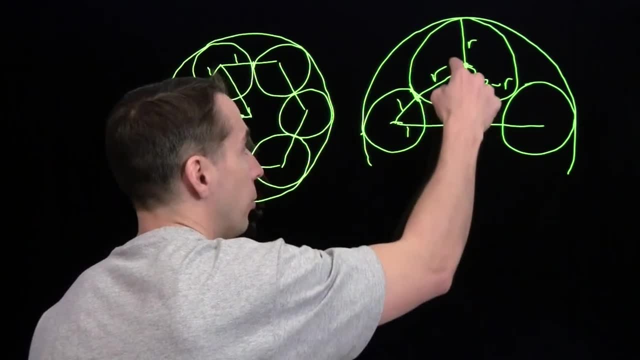 This is r, And then this right here. well, this is one, And we found before that this is one as well. So we've got a right triangle. We've got our classic geometry problem-solving strategy: Build a right triangle, Use the Pythagorean theorem And that's what we're. 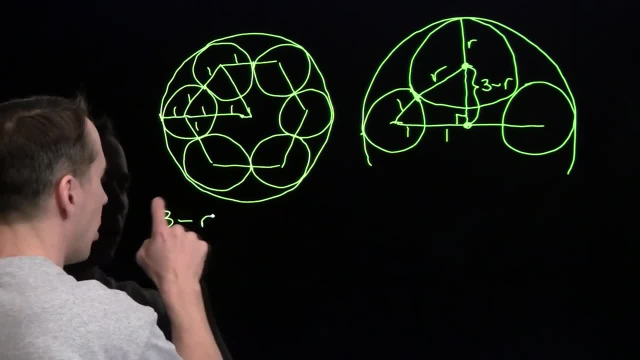 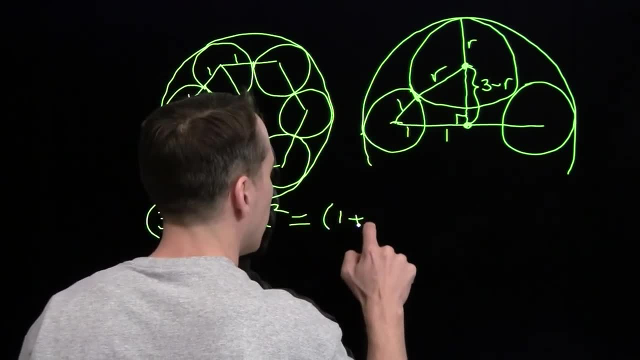 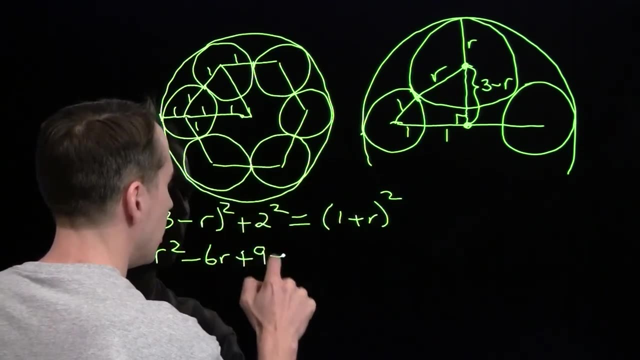 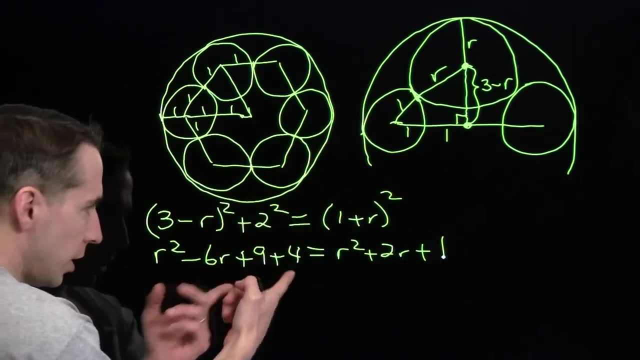 going to do right here. to finish the problem. We have 3 minus r squared plus 2 squared, equals 1 plus r squared. Go ahead and square this out. We have r squared minus 6r plus 2 squared Plus 9 plus 4, equals r squared plus 2r plus 1.. Bring the 1 over here When it's 13 minus. 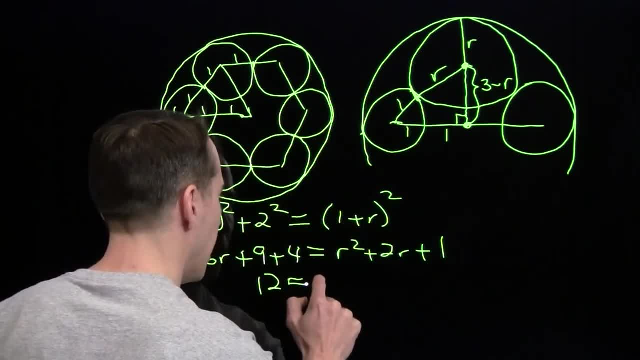 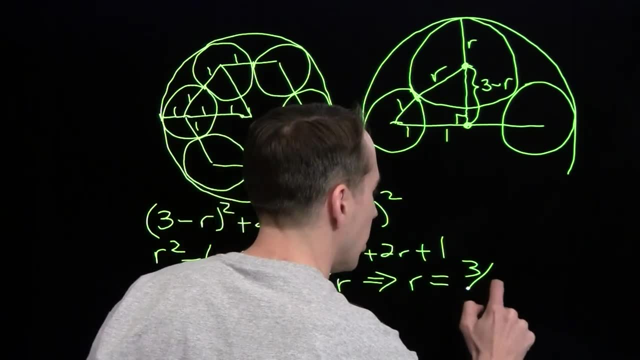 1, it is 12.. Add the 6r over there, We have 12 equals 8r And that gives us r equals 3 halves. We go back to the problem. We find the 3 halves And we're done.